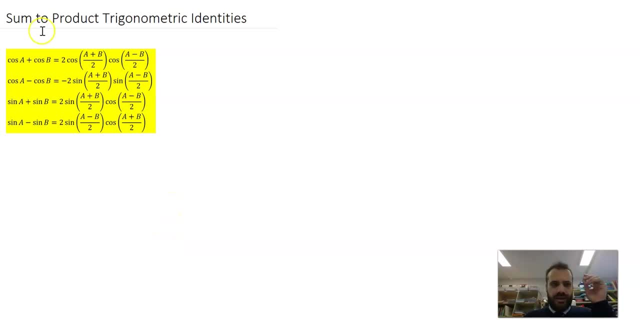 All right, so you already know what the product sum trig identities are. These are the sum product trig identities and you can see the four here. Now deriving them is really, really straightforward. We take the product sum trig identities and we sub in two different things. I'm going to derive: 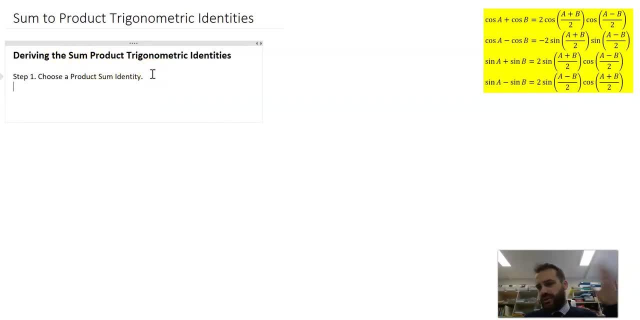 the sum product trig identities. I'm not going to do all four of them, I'm just going to do one, and you can fill in the gaps after that. So step one: choose a product sum identity. So here are my product sum identities, and let's just choose the first one and deal with that one. So step two. 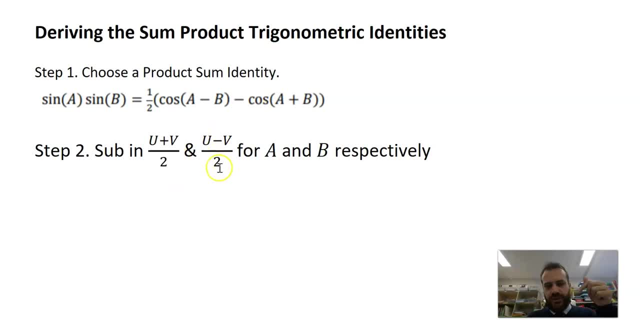 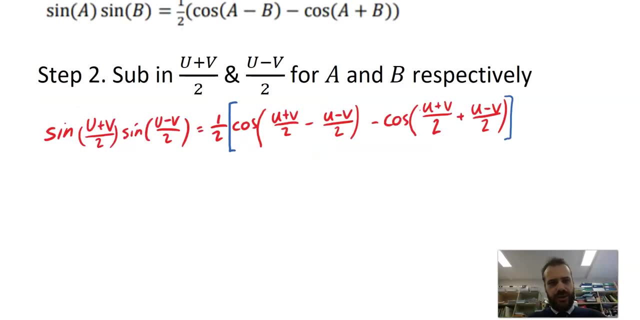 here I'm going to sub in u plus v over 2 and u minus v over 2 for a and b respectively. And don't worry about why, Let's just trust the process. You can see. I put u plus v over 2 for a and u minus v. 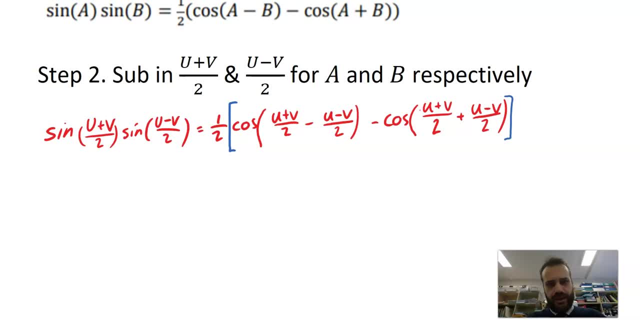 over 2 for b. and then I've done the same here, here, here and here. Now cast your eye over this bit: u plus v over 2 for a and u minus v over 2 for b. Now cast your eye over this bit: u plus v. 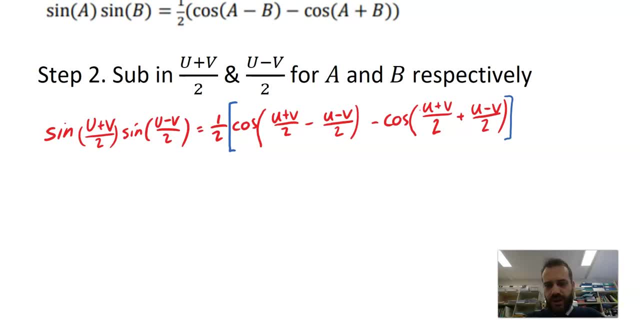 minus u, minus v, both of them over 2.. So because they're both over 2, we're going to be able to subtract those two fractions. Because they're both over 2, we're going to be able to add those two. 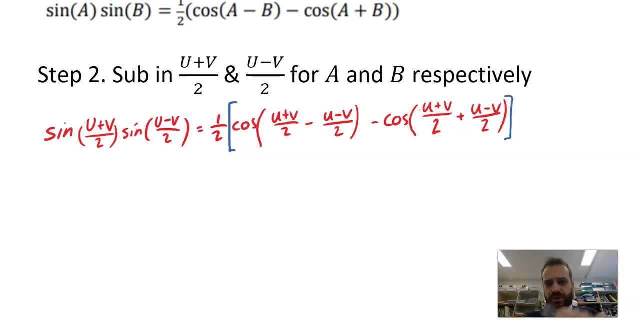 fractions together, And when we simplify it, some of these u's and v's are going to cancel out in some way. Do this next bit in front of you so you can see what I'm doing: u minus u, the u's will. 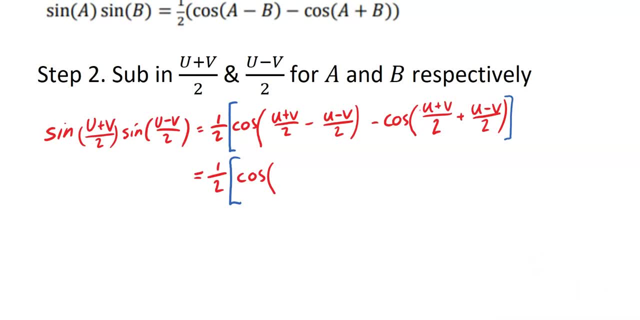 cancel out v minus minus v. that'll give me 2v, but it's going to be 2v over 2, and 2v over 2 is just going to be v. So all of that junk there just becomes v. And then here we get minus cos. 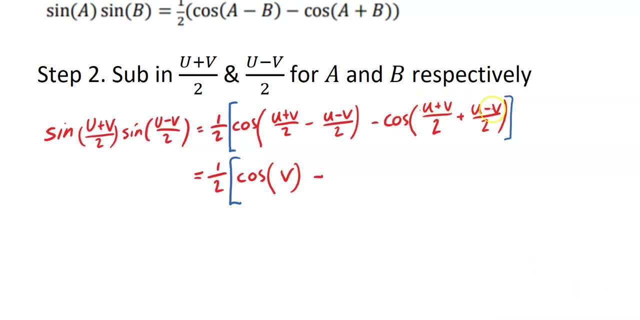 and then u plus v plus u minus v, So u plus u would be 2u. Let's keep that in our head for a second. And v minus v- the v's are going to cancel out, So I'm going to end up with 2u over 2,. 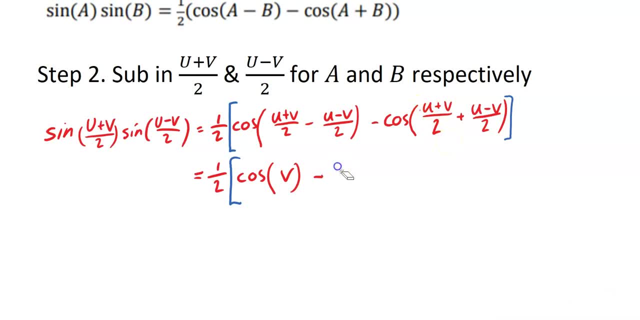 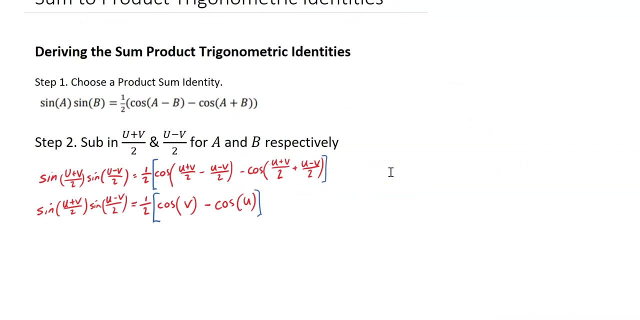 which is just going to be u. And so now we have this neat little thing here that says that sine u plus v over 2, sine u minus v over 2 equals half cos v minus cos u. Finally, traditionally with this we don't leave that half there. Instead, we divide both sides by a half, which is the same. 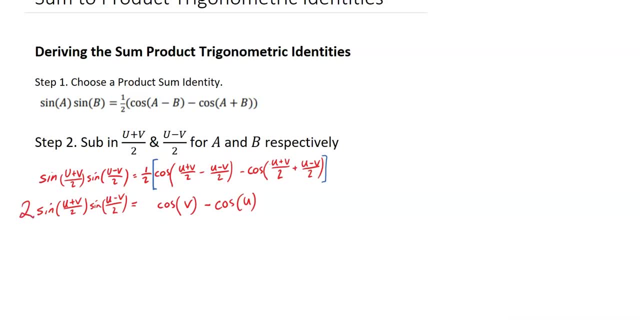 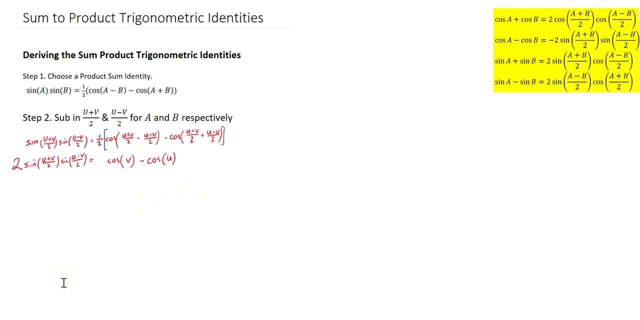 as multiplying both sides by 2, which leads us to this result: 2 sine u plus v over 2, sine u minus v over 2 equals cos v minus cos u, And that is one of our sum product identities. Now, if you take a look at it, you might not recognize it on our list of four here. 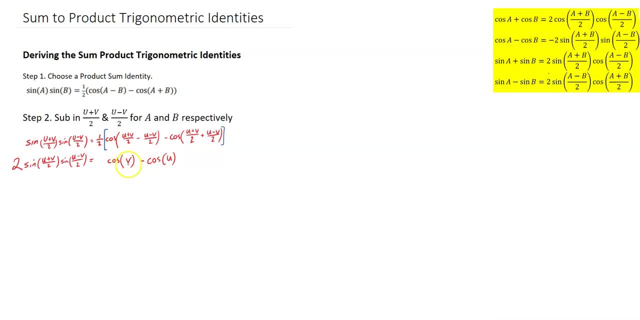 and you're right. I've used the letter u instead of the letter v, instead of a and b. I used u and v because I didn't want to confuse matters here, But also, if you actually take a look at it, it doesn't look like any of these. 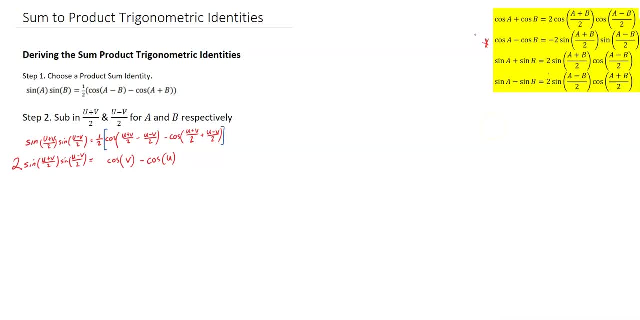 But it's actually this one right here. So I'm just going to rearrange it a little bit, and I'm going to do that by moving this to this side, moving that to that side, or adding them to both sides and then adding that one to this side or subtracting that one from 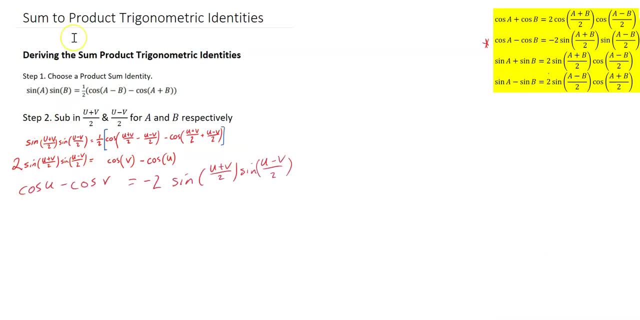 both sides as well, And it's going to look something more like this now: Just moved everything to the other side and you can see we have cos u minus cos v, which is cos a minus cos b, and we have negative 2 sine u plus v over 2, which is cos a minus cos b, which is cos a minus cos b. 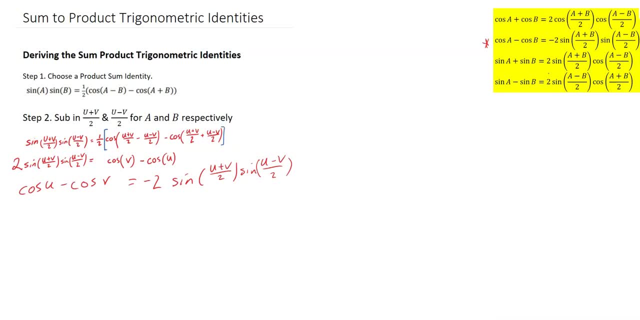 over 2, sine u minus v over 2, which is exactly this with u's and v's instead of a's and b's. Okay, you can derive the other three, this one, this one and this one, in exactly the same way. 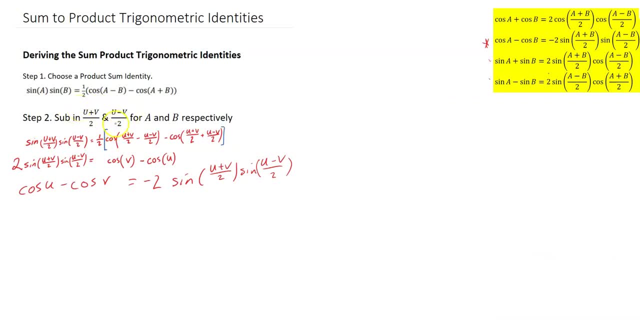 just by summing in u plus v over 2 and u minus v over 2 into the other three product sum identities. Now, of course, the question now is: now that we know that it works, and now we know where it comes from, what are we going to do with it? 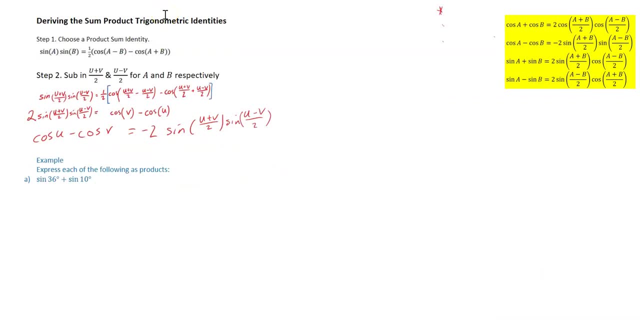 Well, what you're going to do is express a sum of trig functions as a product of trig functions, And it's going to be as simple as taking a look at our sum sine 36 degrees plus sine 10 degrees, looking for our identity, this one right here, sine a plus. 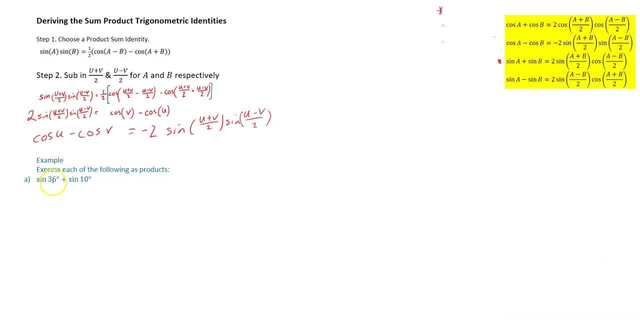 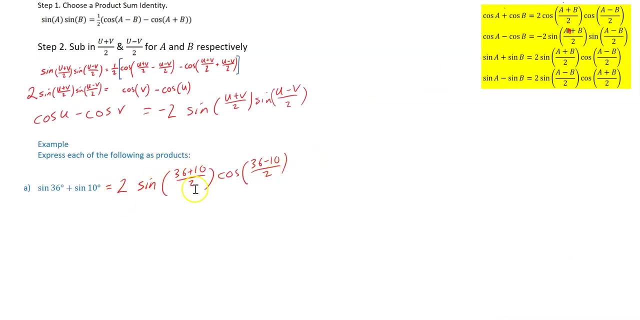 sine b and then subbing in our values 36 and 10 for a and b, what I originally called u and v. when I was working through my Shall, we Epsilon, Epsilon derivation- Subbed in 36 and 10,, 36 plus 10, 36 minus 10, and I'm going to divide them by 2,. 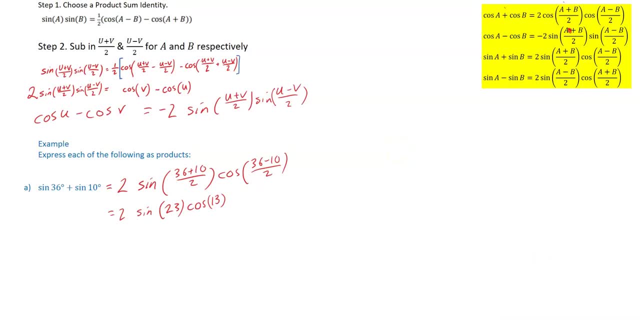 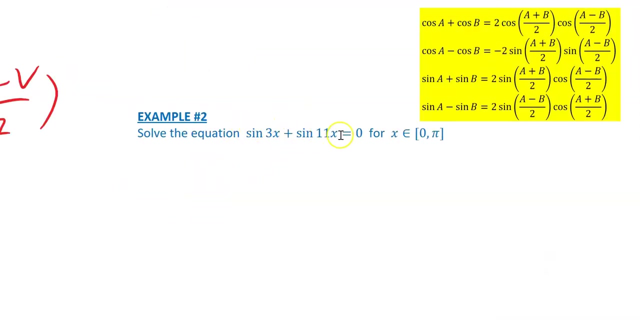 and that's the end. It's two lines are working. That's it. That's one thing that you can do with these. Now, why would I want to write a sum of trig functions as a product of trig function? Well, there's a great reason. Let's try to solve this equation. It's a trig function plus another. 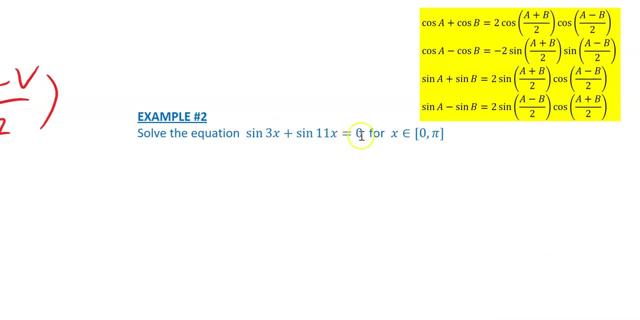 trig function and, importantly, it's equal to 0.. Now, this is a sum. If I were to write it as a product, I'm going to have two trig function products and that means they're multiplied together, right? And if two things are multiplied together and they're equal to 0, the null factor 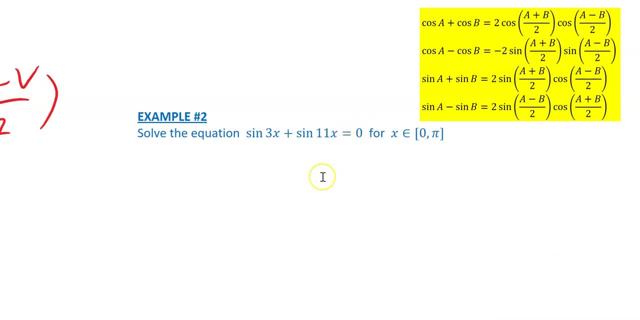 law tells us that the one or the other must be equal to 0. So that's a great reason to be able to do this Now. looking through my for some product identities, I see this as a sine- something plus sine something else. So 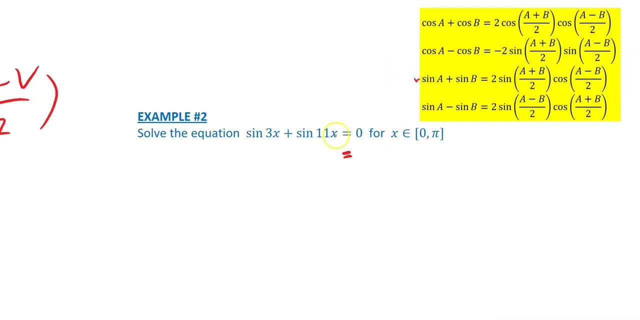 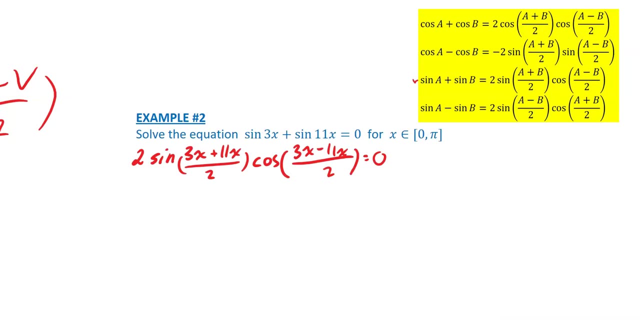 I'm going to have to use this one again and I'm just going to sub in 3x for a and 11x for b, and away we go. Subbed that in Now that 3x plus 11x will be 14x divided by 2x 7x. 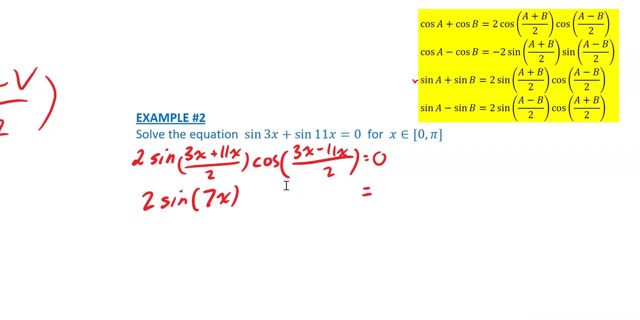 That will be 3x minus 11x over 2,, which is negative, 8x over 2,, which is negative, 4x. Good start. What we have now is this: Times: this equals 0.. Therefore, this must equal 0, or this must equal 0. 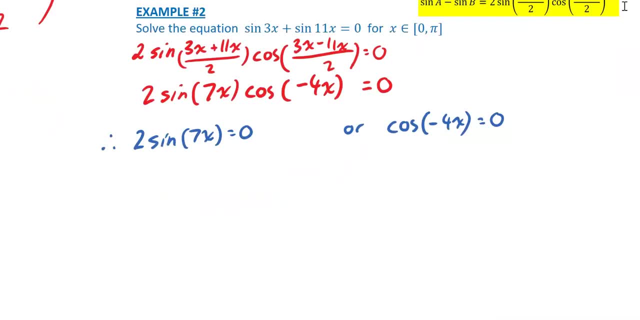 So we've got these setups now, Now that 2 could have come along for the ride wherever, because it's going to vanish anyway, because 0 divided by 2, if I divide 0 divided by 2 will be 0 still. So we can just rewrite that as sine 7x equals 0. 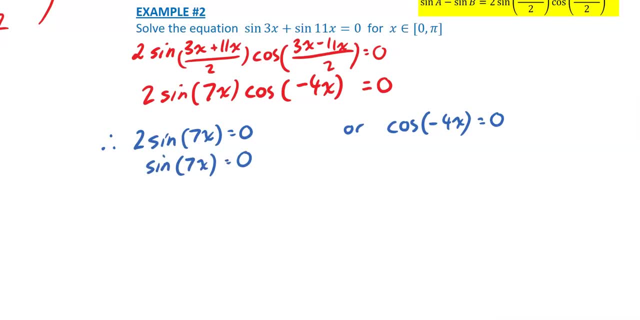 And if sine of something is equal to 0,, then the something must be equal to 0,, or pi or 2pi, or 3pi, or 4pi or 5pi or 6pi, etc. etc. 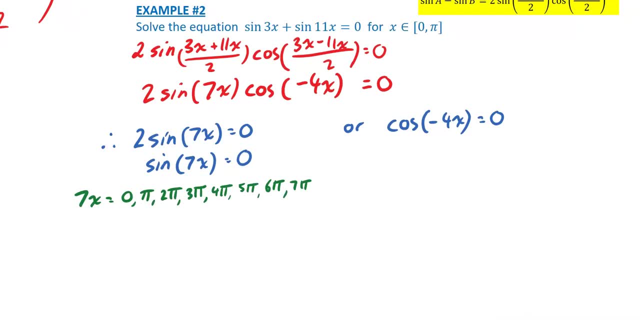 Thinking: wait a minute, why are you going so far? Because the domain is only between 0 and pi, But that's the domain for x, not the domain for 7x. So now I know that 7x is equal to this. 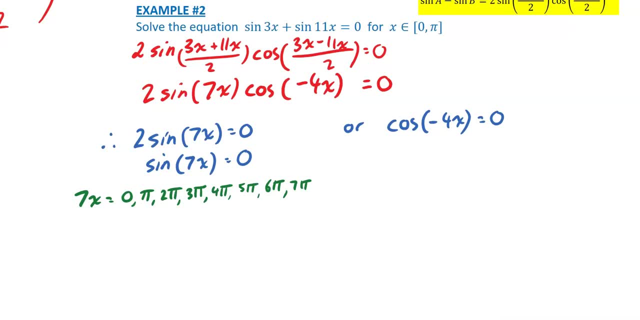 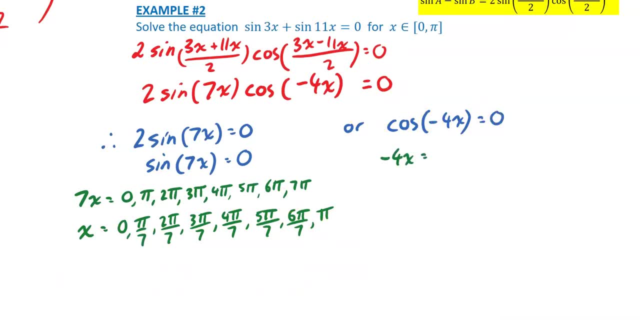 And now I can do the same here, Thinking here to say that negative 4x is equal to pi on 2, 3pi on 2,, 5pi on 2,, 7pi on 2, 9pi on 2.. 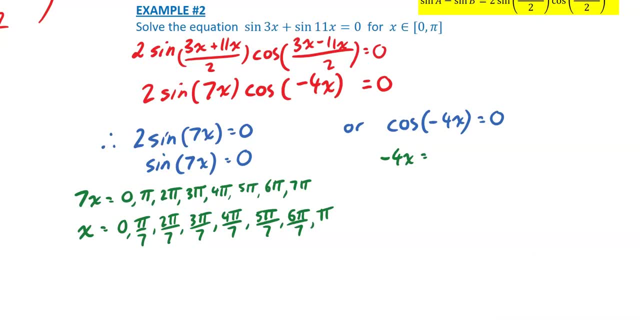 But that would be fine. but when we divide all of those by negative 4, we're going to start getting negative answers, and our domain is between 0 and pi. So instead let's write our solutions here as: negative pi on 2, negative 3pi on 2,. 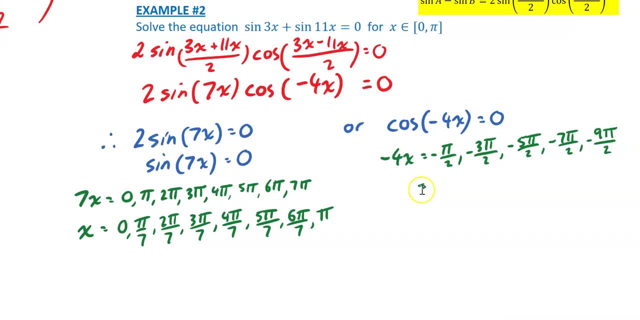 negative 5pi on 2.. We've gone far enough, but let's try that Negative pi on 2 divided by negative 4 will give me positive pi on 8.. Okay, and there's a bunch of answers: Boom, boom, boom, boom, boom, boom, boom. This last one here is a garbage answer. 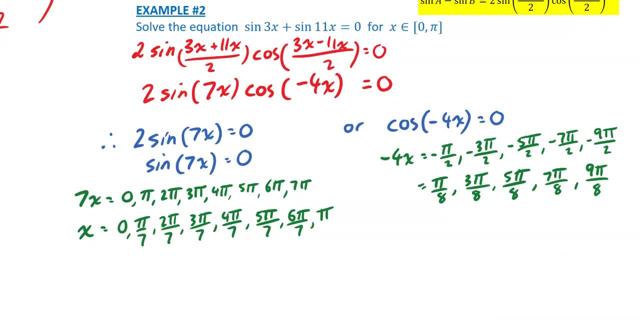 because 9pi on 8 is more than 8pi on 8, and 8pi on 8 would be equal to pi. So we can reject this because it's outside of our domain And we finish with x being equal to. 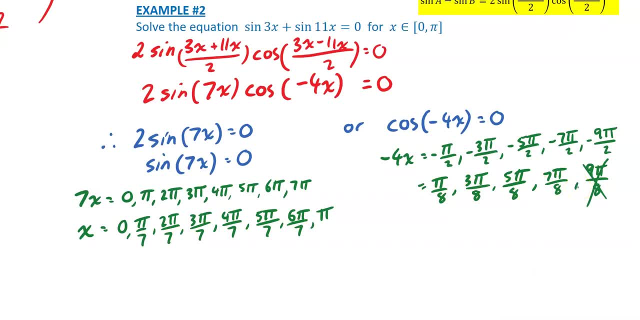 all of these and All of these, All right, so that's pretty good use. If that was all I could use these identities for, I would be pretty happy because it feels like really useful, But of course we could also do some proofs. 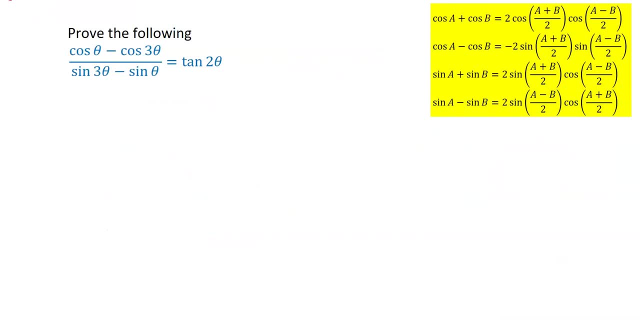 I want to prove this. This stuff on the top of the fraction over this stuff on the bottom of the fraction is equal to tan 2 theta. Now, there's not a lot I can do with tan 2 theta, and usually we want to mess around with the more complicated side than the more simplified side. 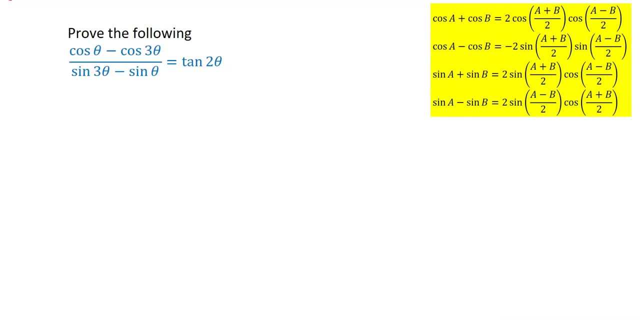 Now we can't really like split this fraction up at the moment, but if we can create products top and bottom of this fraction, maybe some of those products would be equal and we could start cancelling them out. So I see two useful identities for me to use here, So I can use the cos. 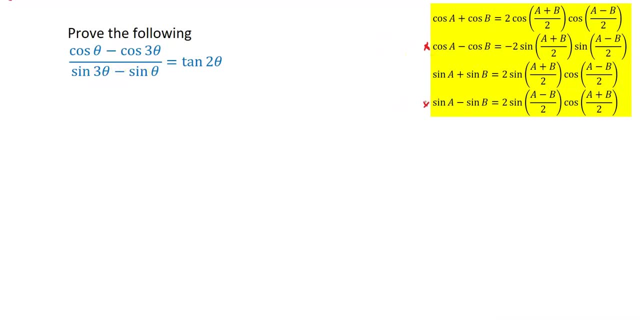 the minus one here and sin the minus one here and I can sub in theta and 3 theta respectively. I think so will lead me to this. Just be aware that on the top side, theta was our a value and 3 theta was our b value, Whereas on the bottom side, 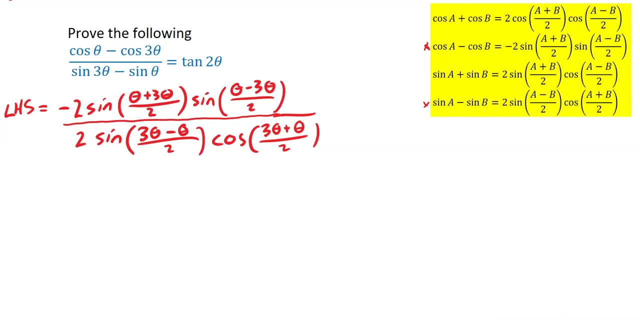 3: theta was our a value and theta was our b value, So they were reversed top and bottom. Okay, from here we can simplify that stuff, Simplify that, simplify that, simplify that We've also got, because this is all a product and this is all a product, I can also get rid of the 2s. 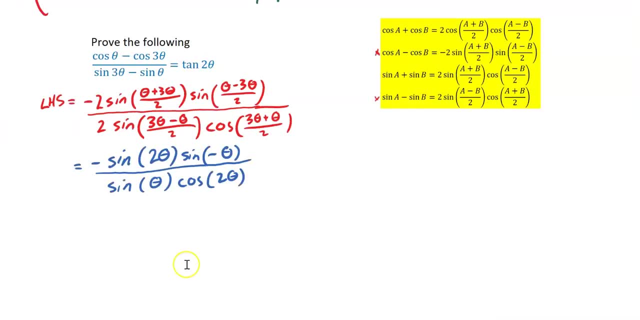 uh, cancel them out and I'll just have a negative up at the top. If you stop and take stock for a second, you should be looking at sin 2 theta and looking at cos 2 theta and saying, well, if it was just that over that, that would be 10: 2 theta and I would be. 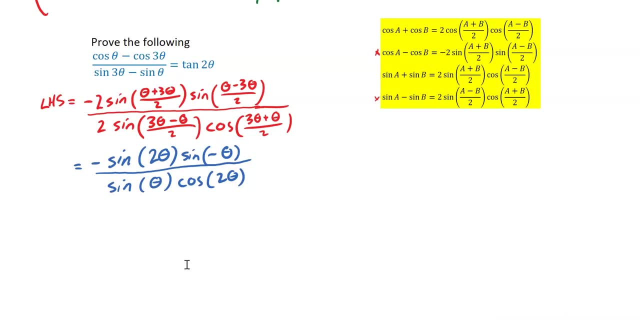 finished, because that's what I'm trying to prove. So it's this thing and this thing that are in the way, and you should notice that they look really similar. but sin, negative theta and sin theta are not equal, But lucky for us. 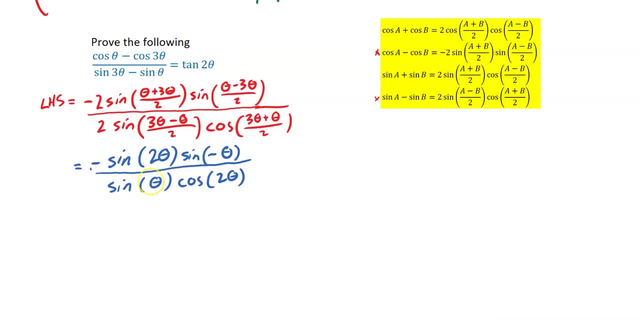 negative, sin, negative theta and sin theta are equal If you think about it. that's sin theta. there is the y coordinate, uh, that's theta. This would be sin of negative theta, the y coordinate of that thing. Now, if we take the negative of that, we'd be taking a negative.